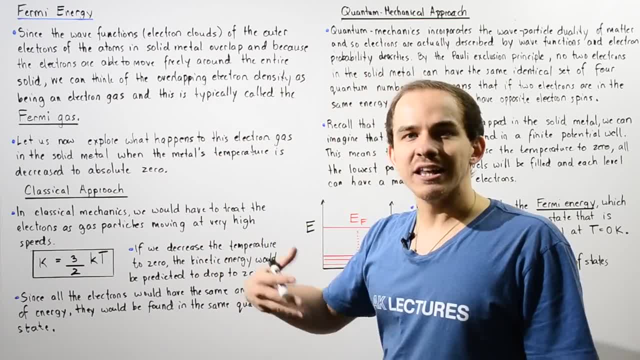 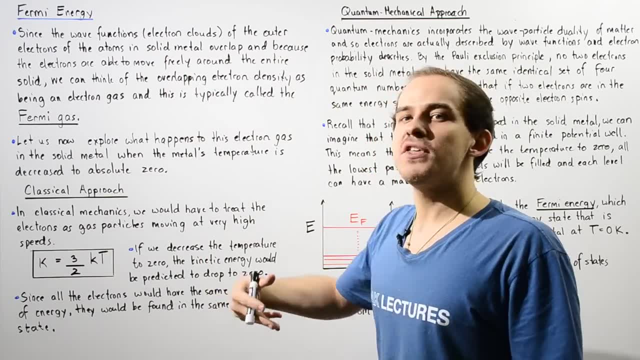 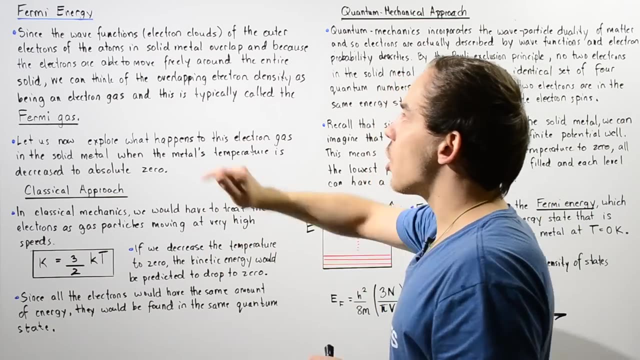 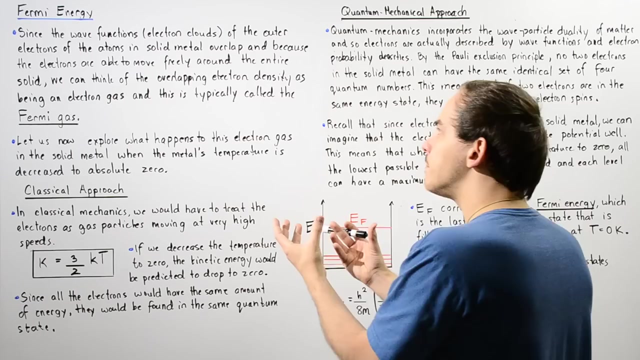 So since the wave functions or electron probability densities, also known as electron clouds, of the outer electrons of the individual atoms inside the solid metal overlap, and because the electrons are able to move freely around the entire solid metal, we can think of this overlapping of electron density distributions. 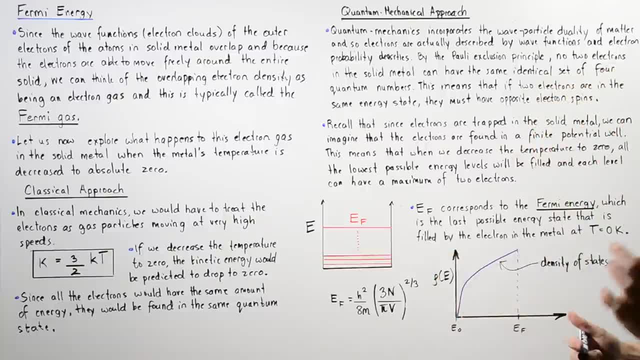 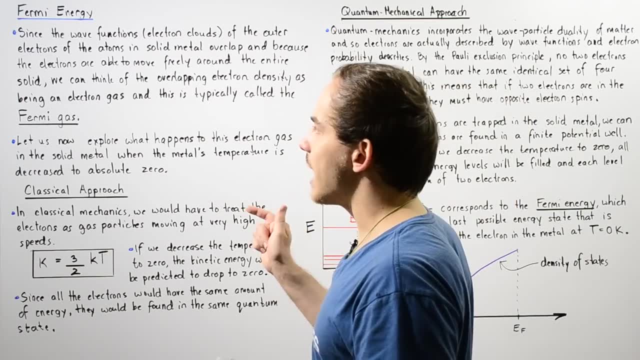 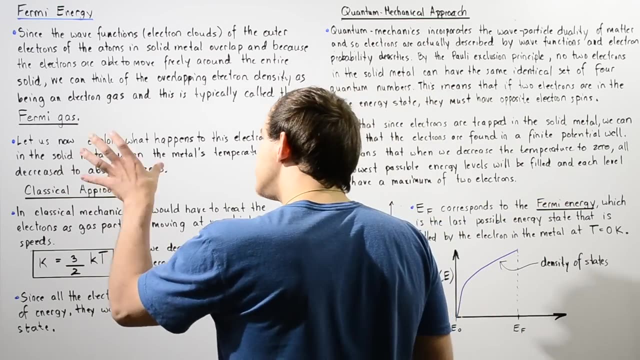 as being an electron probability densityינ gas, and this is typically called the Fermi gas. So basically, in one way, we can think of our electrons inside our solid state, inside our solid metal, as being a gas. Now, let us now explore. 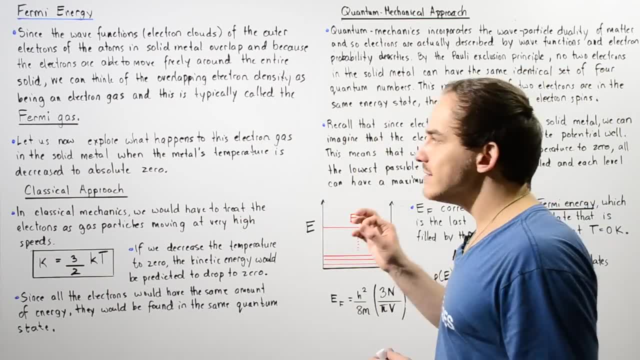 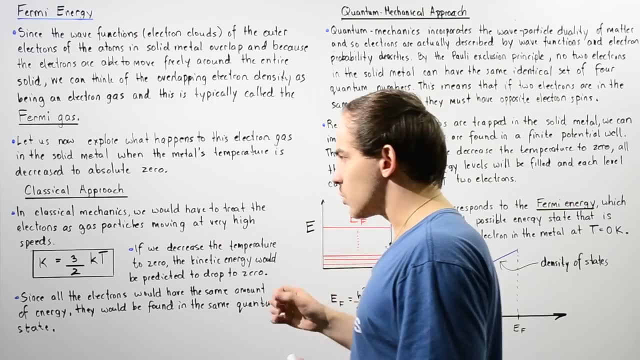 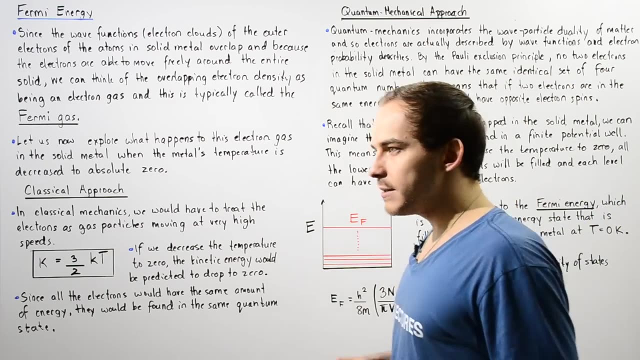 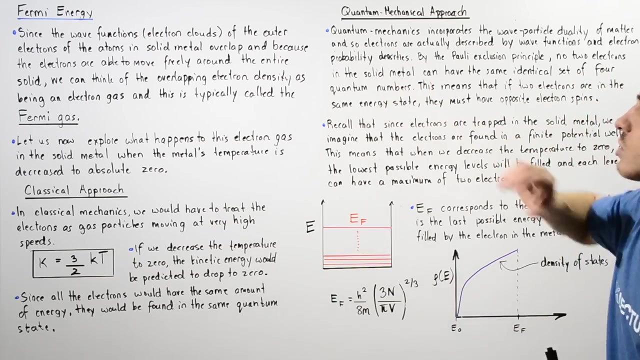 what happens to our electrons inside our solid metal when the metal's temperature is decreased to absolute zero. So this is absolute zero, given in Kelvin. so zero Kelvin. And let's begin by examining what classical mechanics will tell us about this situation, and then we're going to 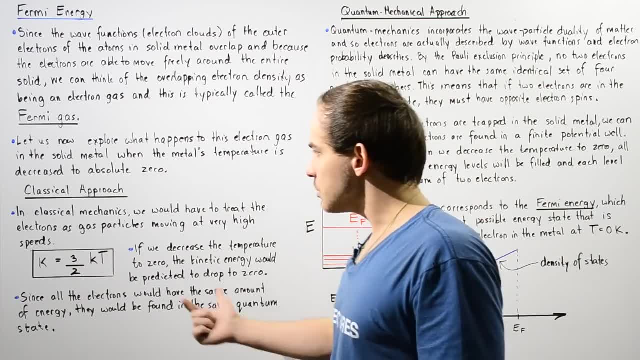 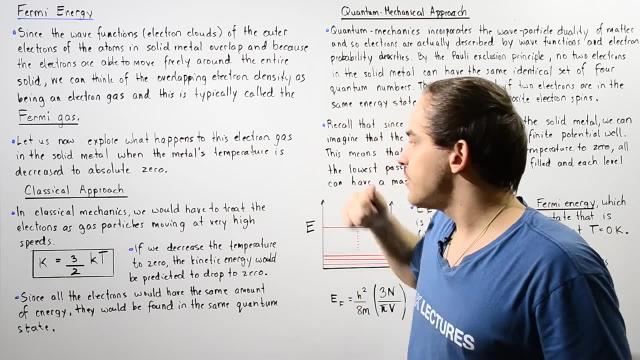 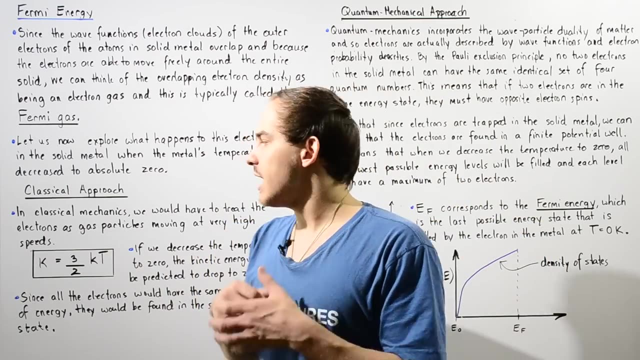 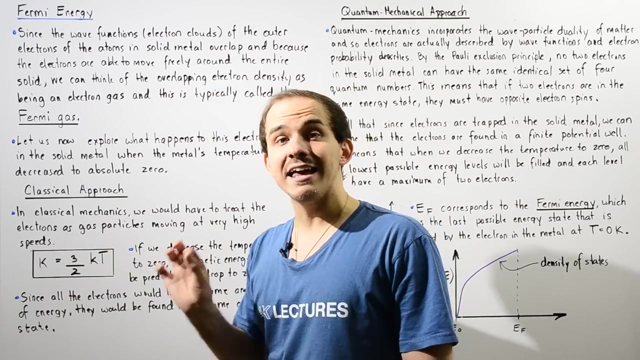 discuss the quantum mechanical approach. So in classical mechanics, since we're discussing an electron gas, we can think of our electrons as being idealized, ideal gas particles that are moving with very high velocities, with very high speeds. Now, this is the equation that gives us our kinetic energy of the individual electron. 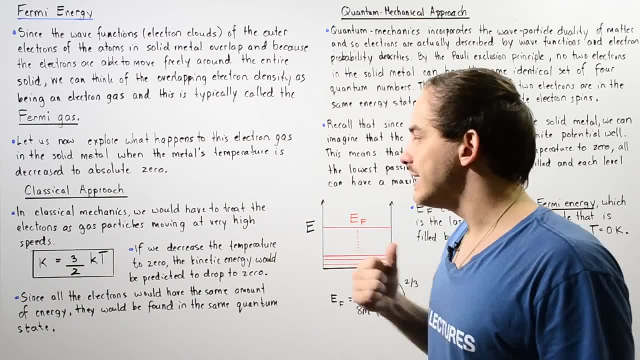 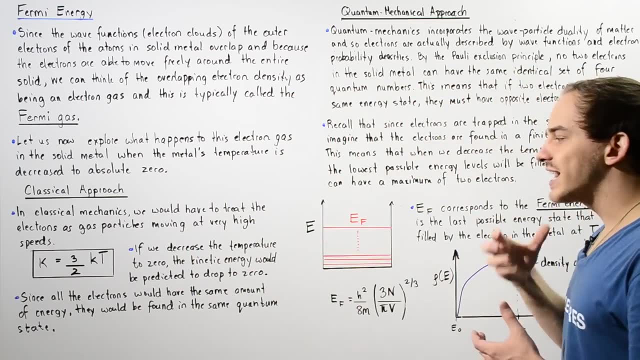 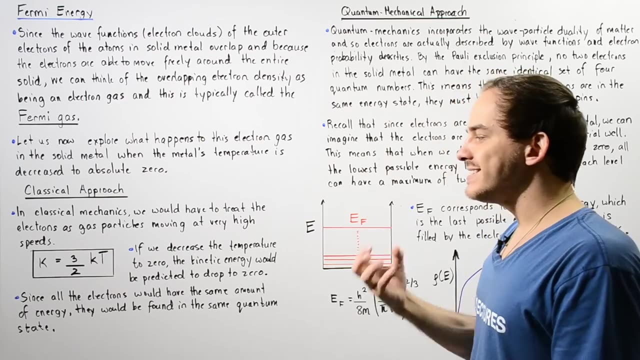 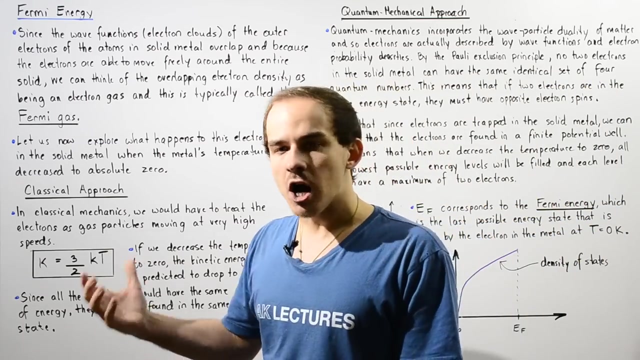 and we see that it depends on the temperature given in Kelvin. So if we decrease the temperature of the entire system to zero, we see that the kinetic energy of each electron would essentially go to zero and the electron would cease to move Now, since all electrons would have the same exact energy and energy of zero joules in. 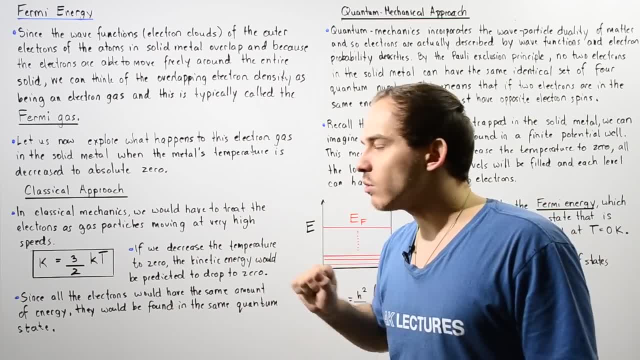 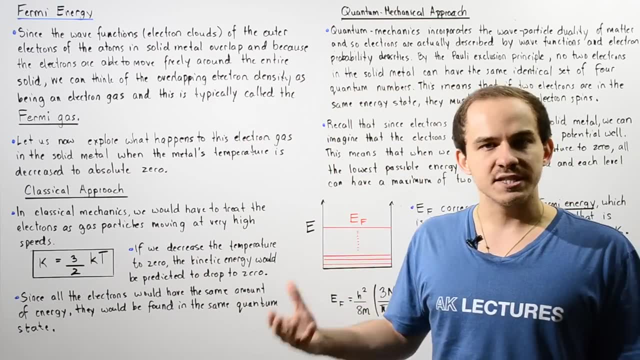 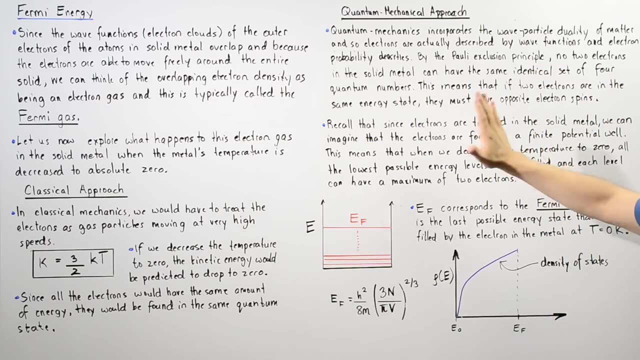 such a case, that would imply that our electrons and all the electrons inside our solid metal would be found in the same quantum state, and we know that that actually cannot take place as a result of the kinetic energy, The Pauli Exclusion Principle- which comes from quantum mechanics. 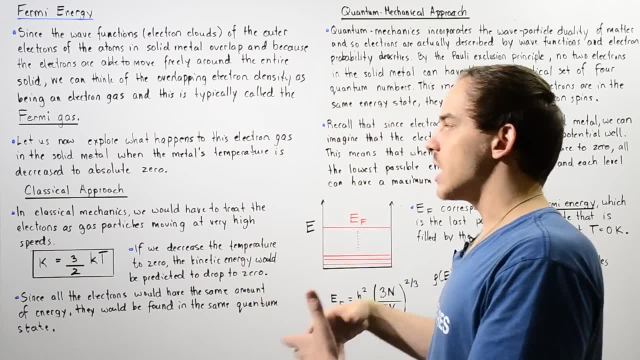 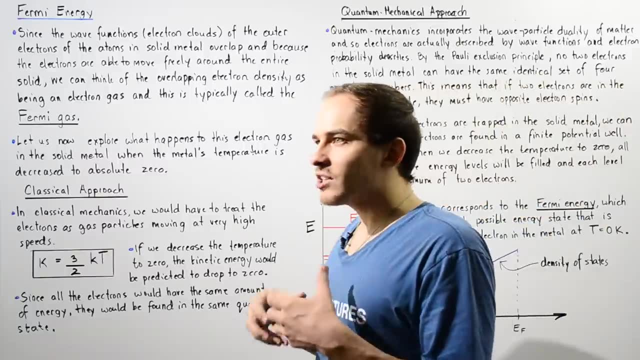 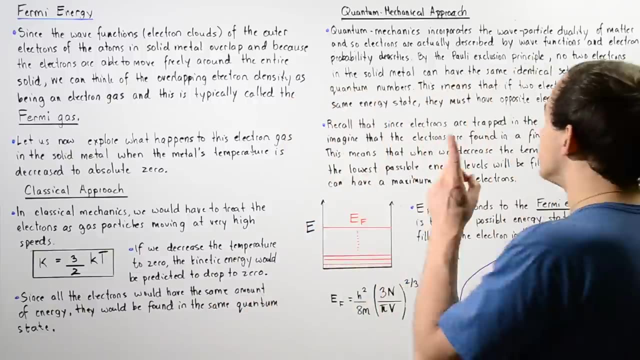 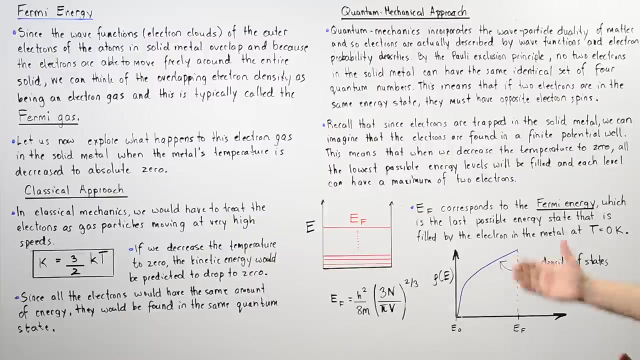 So we see that this approach does not actually give us a valid result. Now let's take the quantum mechanical approach. So recall that quantum mechanics basically incorporates the wave-particle duality of matter, that is, electrons are actually described not as particles but as waves, using equations. 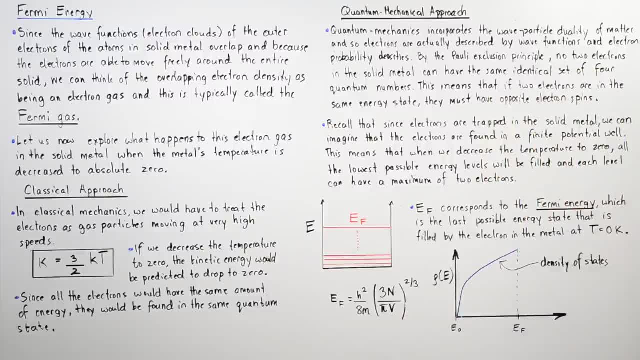 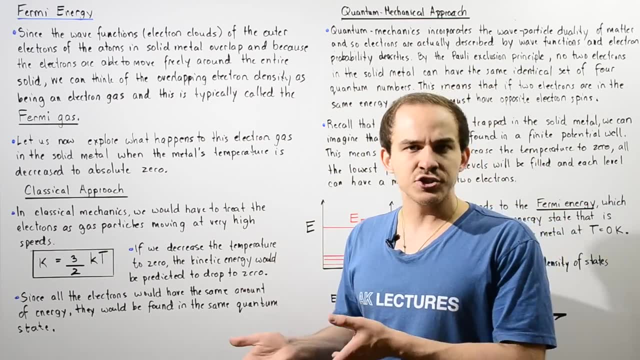 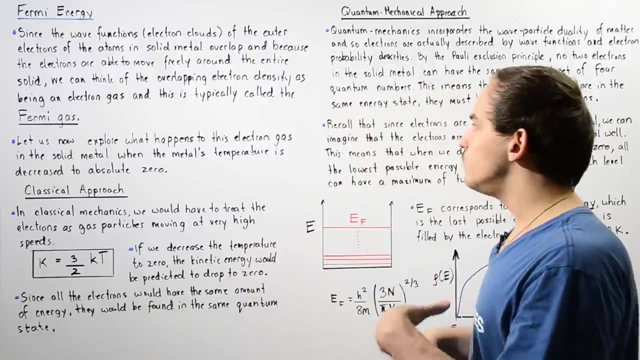 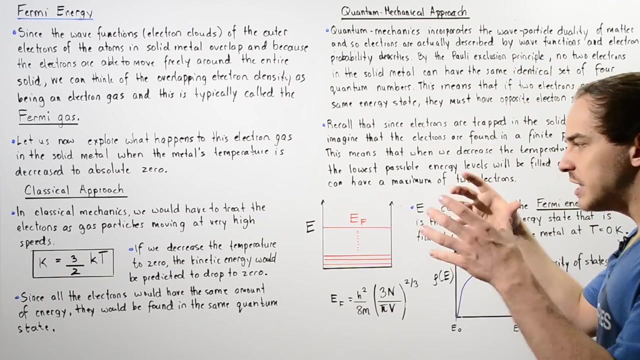 we know as waves. So in quantum mechanics we can use the Schrodinger's equation to solve for the wave-function of any particular electron within any particular atom, and we can use those wave-functions to determine what the electron probability distribution is, which gives us the likelihood of finding. 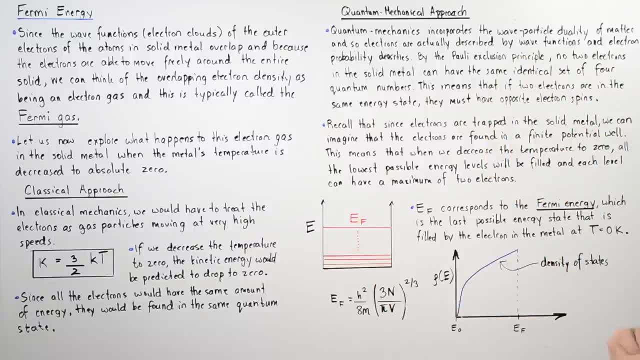 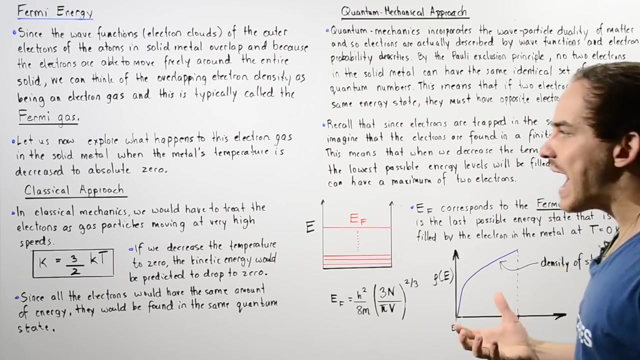 our electrons within some given region. Now, So by the Pauli Exclusion Principle, no two electrons in any solid metal can actually have the same identical set of quantum numbers, and this means that if two electrons are in the same exact energy state, that means they must have opposite electron spins. 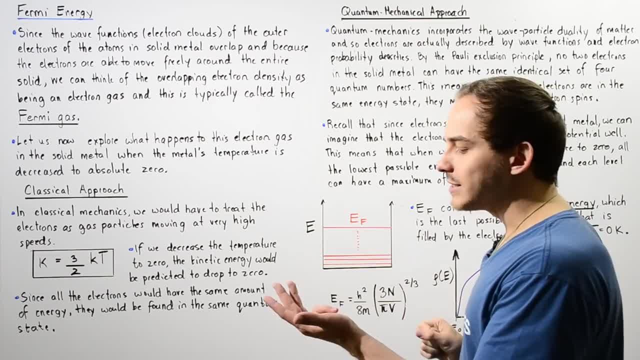 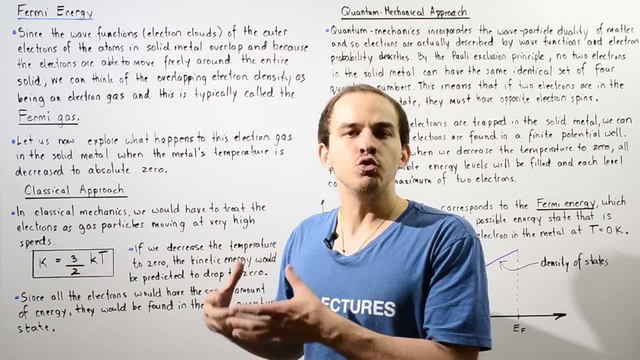 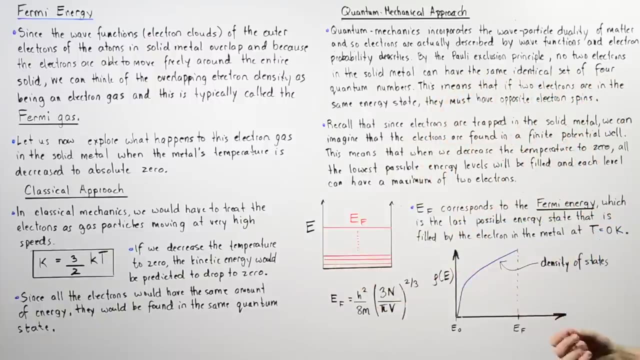 So if two electrons have the same principle- quantum number, orbital quantum number and magnetic quantum number- that means they must have two different electron spins. One has a positive, one half, and the other one must have a negative one half. Now, as we mentioned earlier, recall that since electrons are trapped in the solid metal, 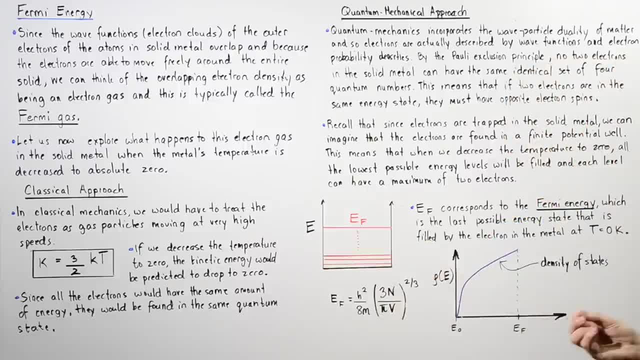 we can imagine that the electrons are found inside a finite potential, well also known as a rigid box. This means that when we decrease the temperature of our solid system of the rigid box to a temperature of absolute zero, all the lowest possible energy levels that the electrons 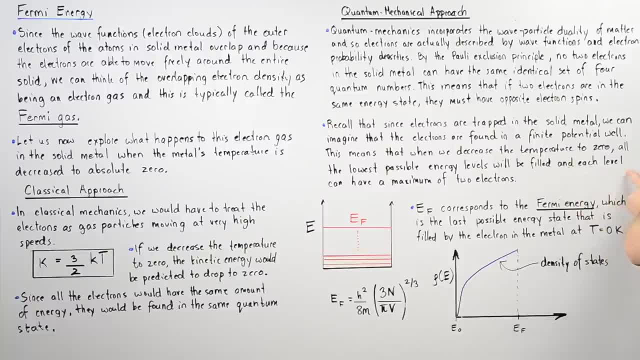 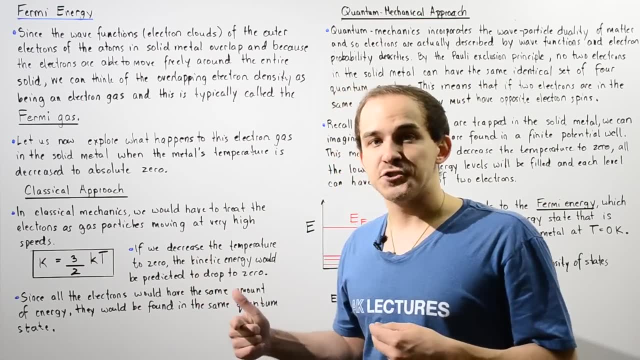 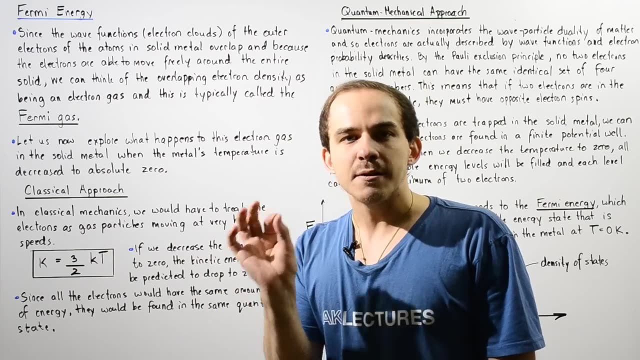 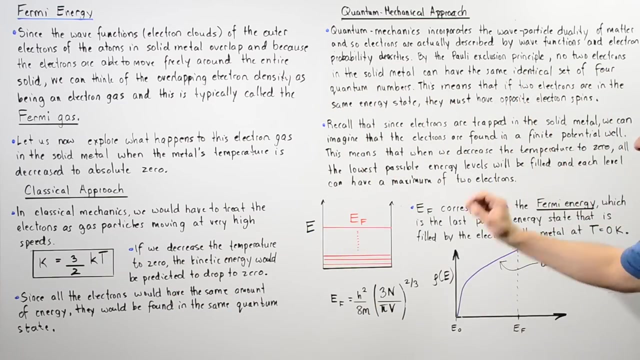 can actually take will be filled, and each level will only have a maximum of two electrons which each have opposite spins. So As soon decrease our temperature to absolute zero, quantum mechanics tells us that the electrons will not have an energy of zero, but it tells us that every electron will basically drop. 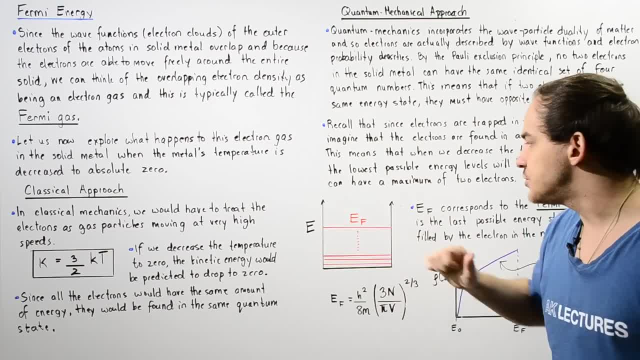 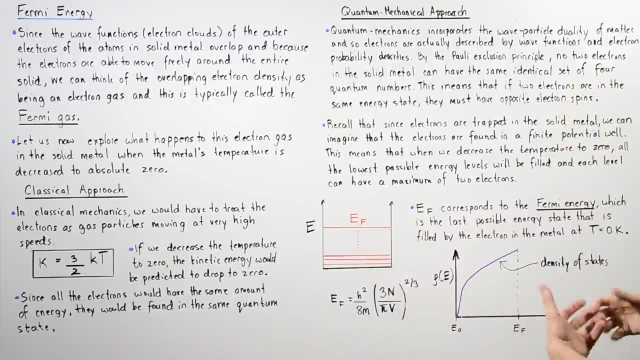 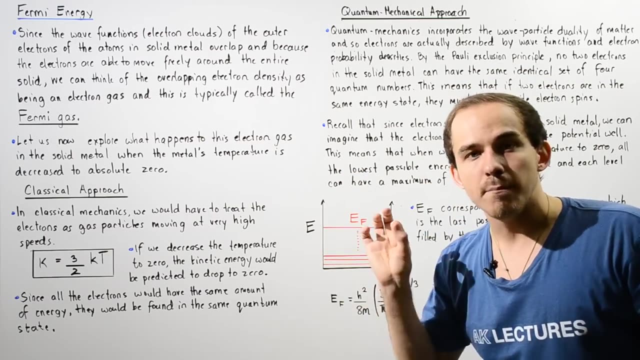 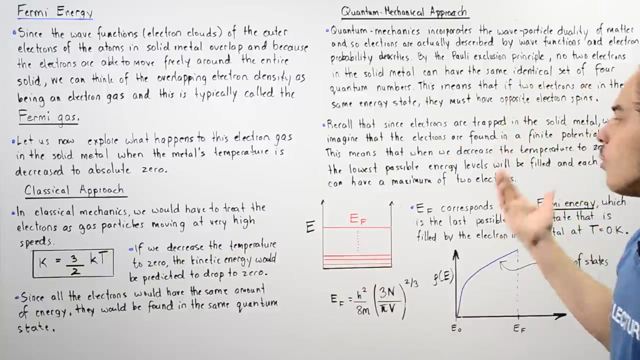 down to all the possible lowest energy states. So, if this diagram represents our rigid box, our finite potential, well, which basically represents our metal, our solid metal, we'll see that two electrons, or a maximum of two electrons, can go in each one of these energy levels, as per the Pauli exclusion principle. 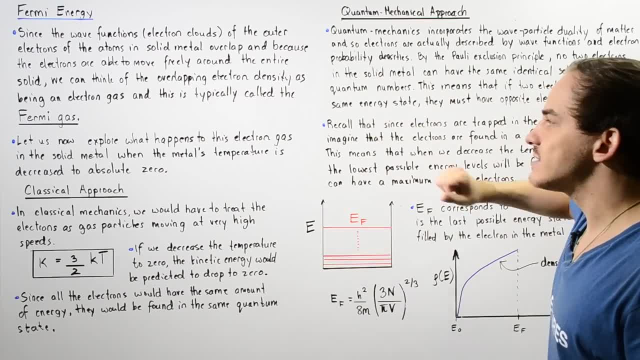 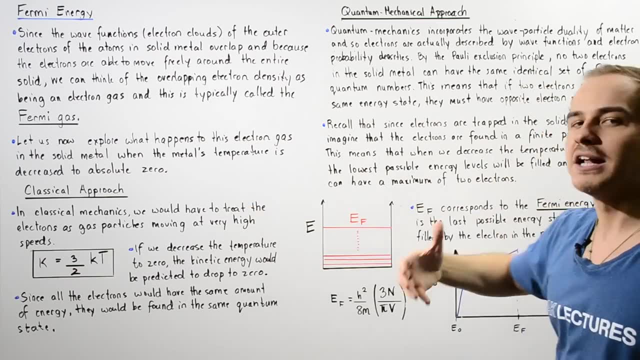 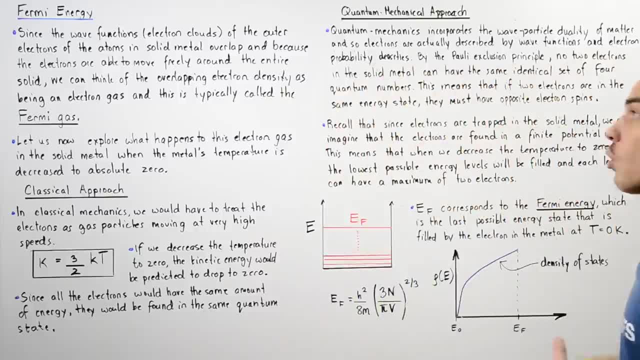 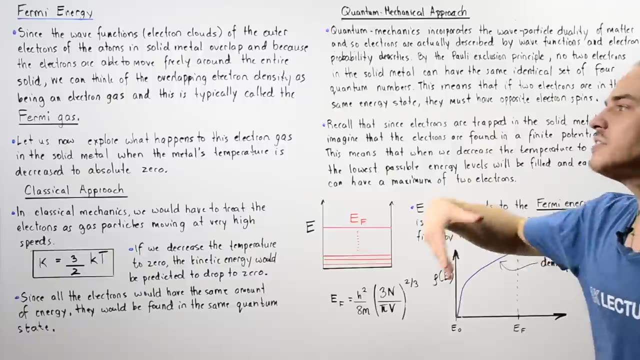 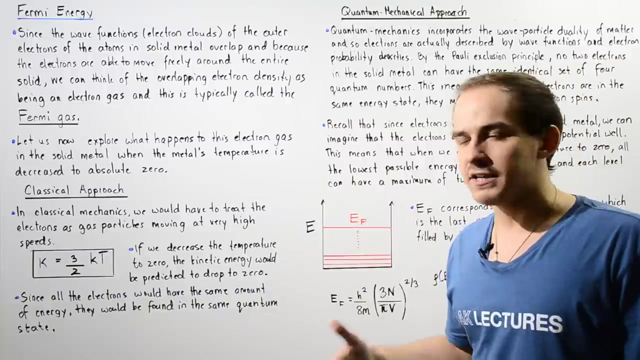 E-quantum state level is known as the Fermi energy or the Fermi level. So the Fermi energy corresponds to the Fermi energy level, which is the last possible energy state that can be filled by the last two electrons inside our solid metal at a temperature of zero Kelvin, at a temperature of absolute zero. 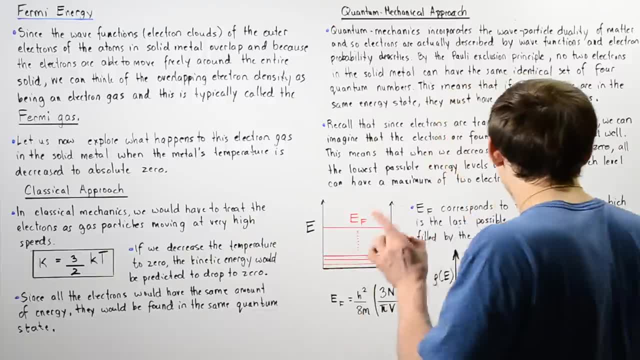 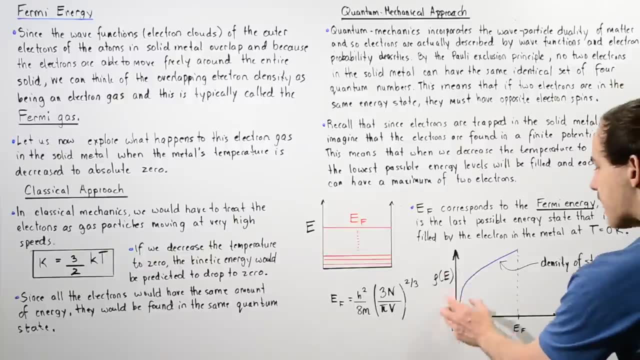 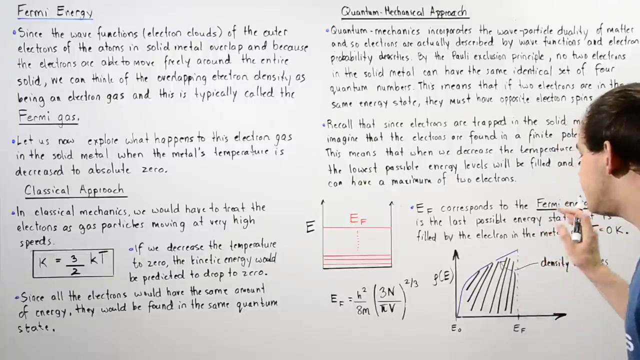 Now we can actually use the density of states function as shown in the following diagram, And if we integrate from our energy of zero to the Fermi energy, we get this entire shaded region. So we basically can calculate what this shaded region is And then we can use this value to. 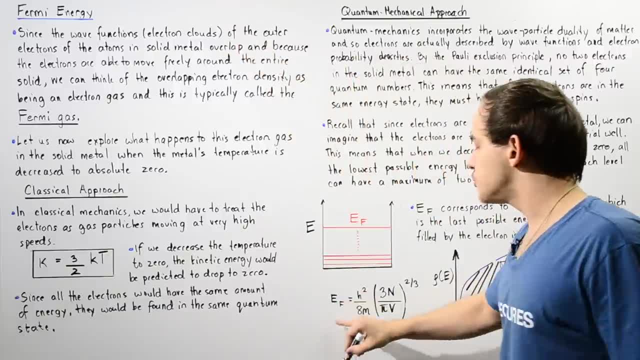 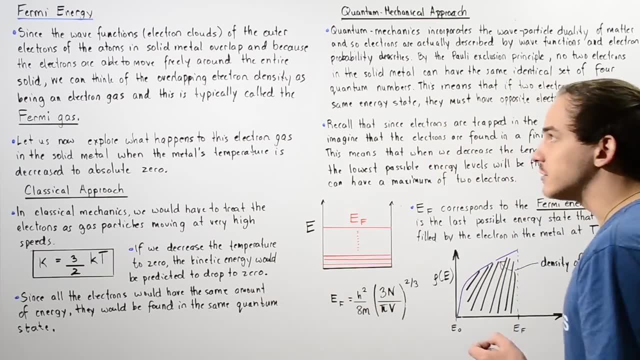 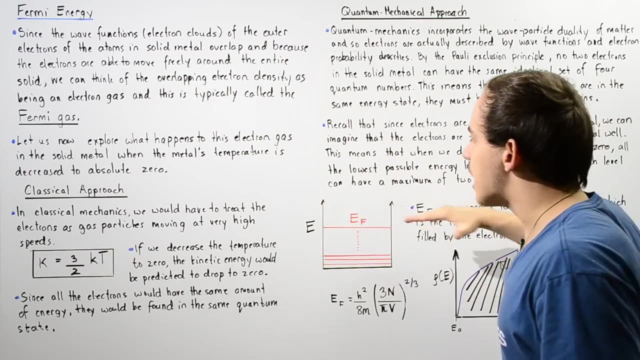 calculate what our Fermi energy actually is. Now we're going to skip the specifics of those steps And we're simply going to give you the end result. So the Fermi energy of our electron, the last possible energy level of our state in. 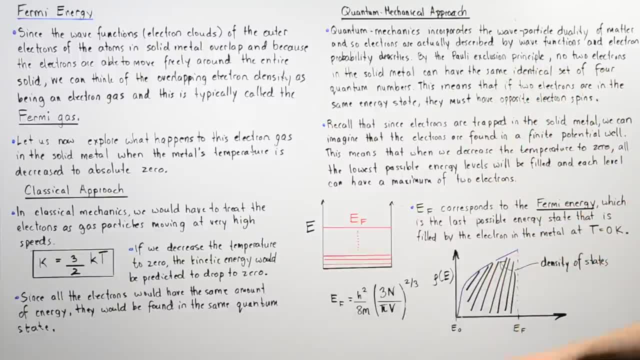 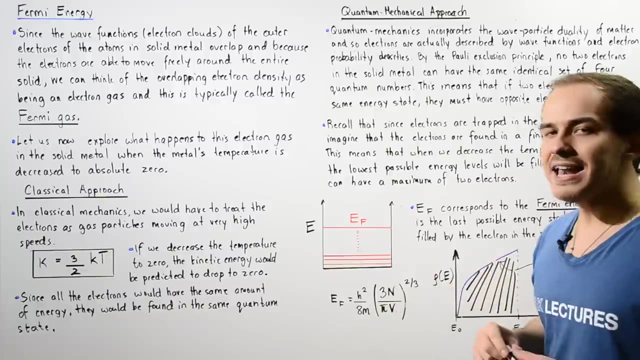 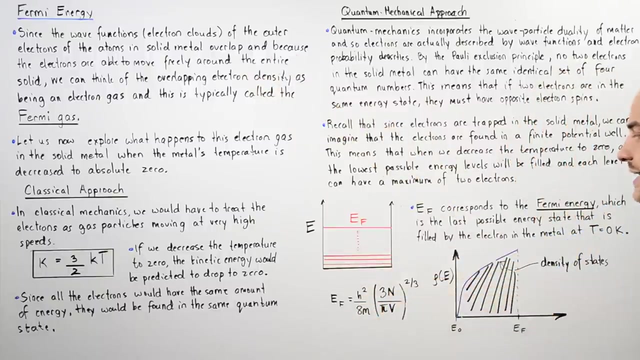 when our temperature is zero inside our solid metal is given by this equation, So and basically gives us the number of our possible quantum states, V as the volume and as in, m is the mass of our electron and ages Planck's constant. So our Fermi energy EF is equal to H squared divided by eight, m multiplied by two, divided by three.